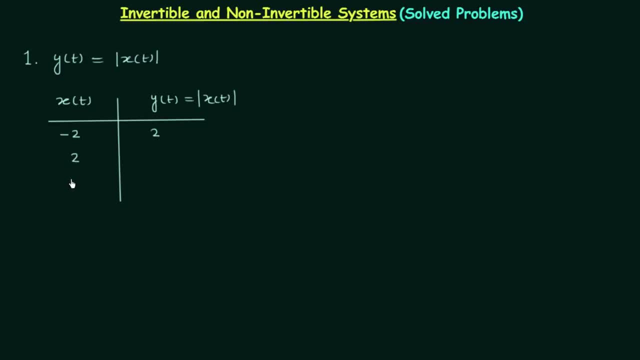 is 2.. Mod 2 is equal to 2 again. Then I will take 2j. Mod 2j is equal to 2.. Then I will take minus 2j And mod minus 2j is equal to 2 again. Therefore, you can see when xt is. 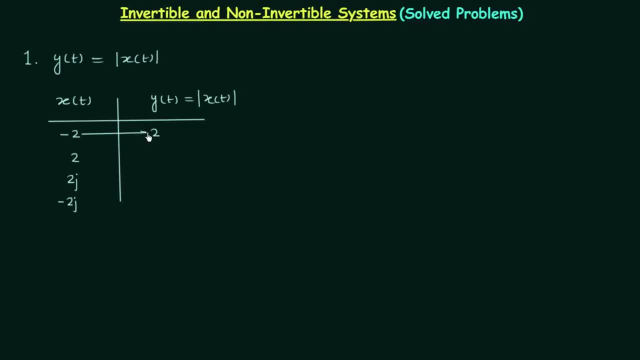 equal to minus 2,, the output is equal to 2.. When xt is equal to 2,, the output is equal to minus 2.. 2, the output is 2. again, When xt is equal to 2j, the output is 2, and when xt is equal. 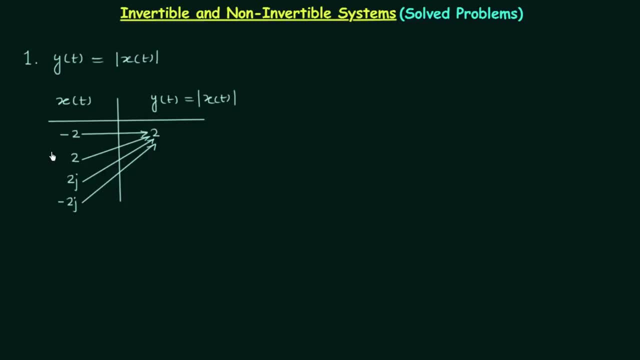 to minus 2j, the output is equal to 2.. So, for 4 different values of input, we have the same value of output. Therefore, there is many to one mapping, and when there is many to one mapping, the signal is non-invertible. The signal is non-invertible and this is our. 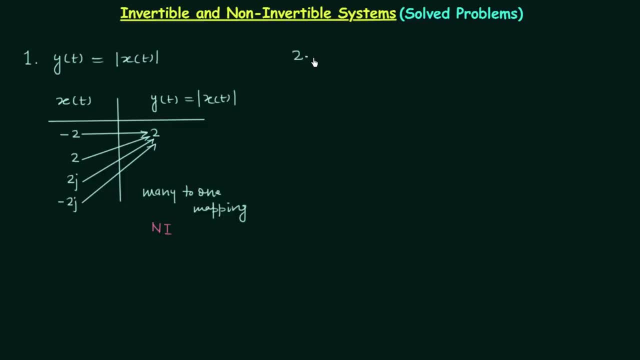 answer. Now we will move to the second problem. The second problem is an important problem. Here yt is equal to sin t multiplied to the input xt. This problem is important because our approach till now will not exactly work here. I will explain you why. First we will 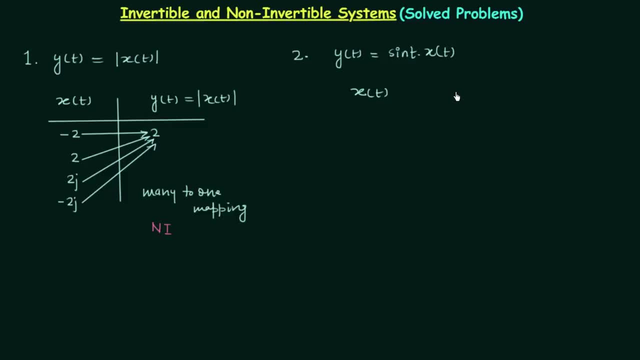 make the table. The first column is for the input. The second column is for the output. It is equal to sin t multiplied to xt. Till now we are selecting numerical values for the input. I will do the same. Let's say xt is equal to 0. So yt will be equal to sin. 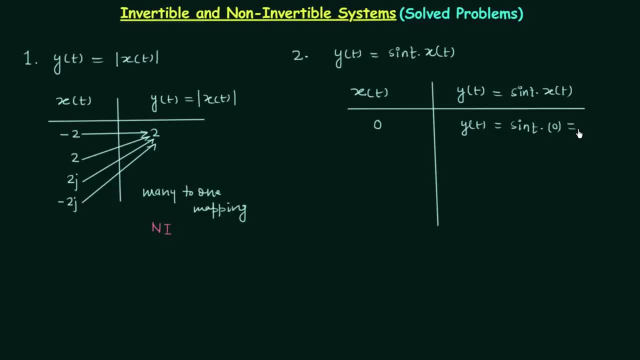 t multiplied to 0, which is equal to 0. So things are fine when xt is equal to 0. We don't know exactly the value of sin t when xt is equal to 0 because we don't know the time instant, We don't know at what time instant. 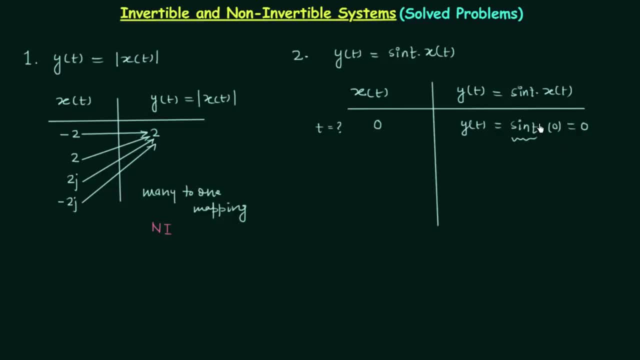 xt is equal to 0. Therefore, we cannot put the time instant at this place and we cannot calculate sin t. That's why I left sin t as it is. But xt is equal to 0. So the overall result will become 0. So in the first case, when xt is 0, yt is equal to 0. There is 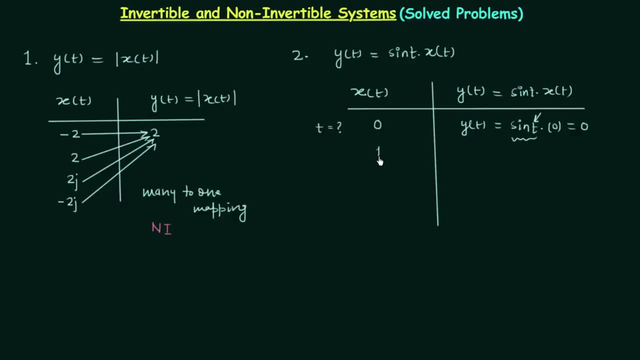 no problem. But now we will take the next numerical value. Let's say it is 1.. So xt is equal to 1 at some time instant which we don't know. So yt will be equal to sin t multiplied by 1, or simply sin t. Now we will take the next numerical value. let's say 2. 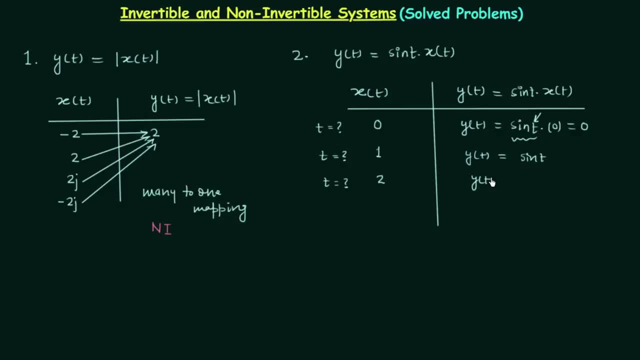 at some time instant, which we don't know. So yt will be equal to 2 sin t. You will say we have three different values of output for three different values of input. Therefore the system is invertible. But you cannot guarantee that sin t is different than 2 sin t. Let's 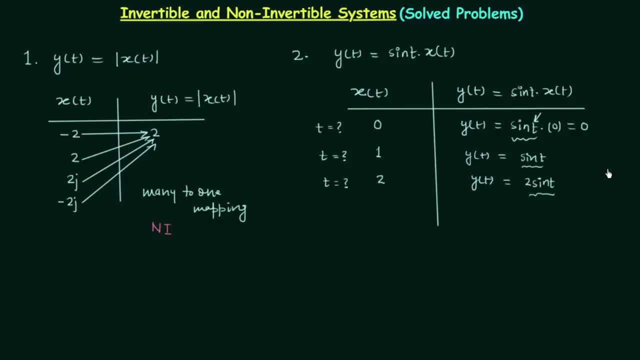 say xt is equal to 1 at the time instant when sin t is equal to 1.. So yt will be equal to 1.. This is something we have assumed. And let's say xt is equal to 2 at a time instant. 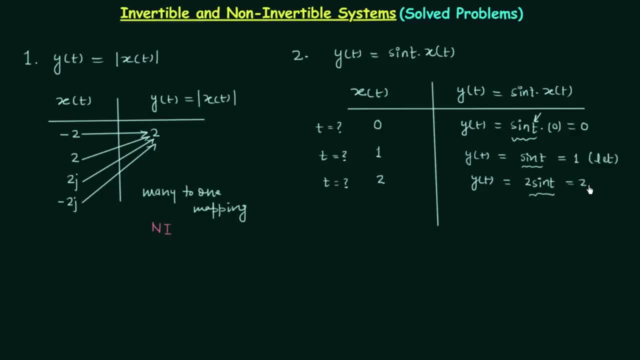 when sin t is equal to 1 by 2.. So it is equal to 1.. And sin t 1 by 2 is also the assumption. So you can see yt is equal to 1 for both xt equal to 1 and xt equal to 2.. So for two different values of input. 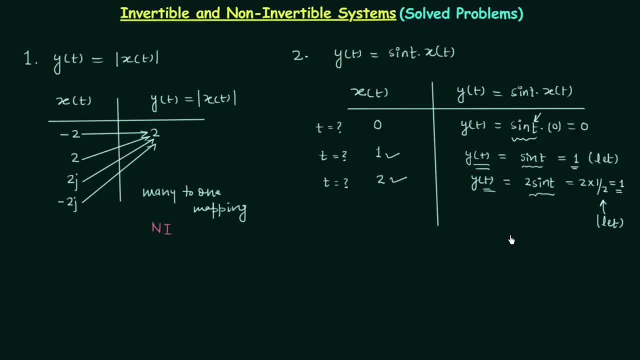 the output is same. Therefore the system is non-invertible. So you can see, you cannot comment exactly about the nature of the system when you take the numerical value. So whenever the problem is little bit complicated, don't select the numerical values as your. 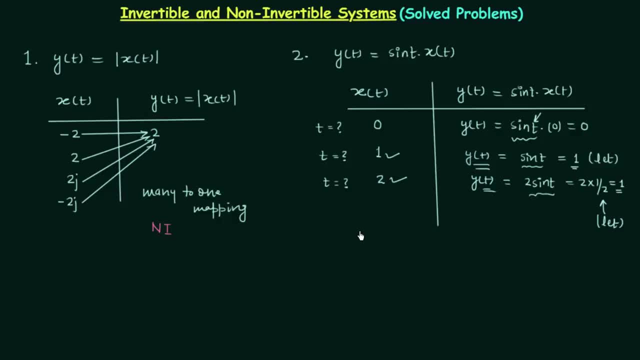 input. You can select the standard signals like impulse and step to solve the question. For example, let's say xt is equal to delta t, which is the unit impulse signal, And for this output, yt is equal to sin t multiplied to delta t And it is equal to 0.. Now how? 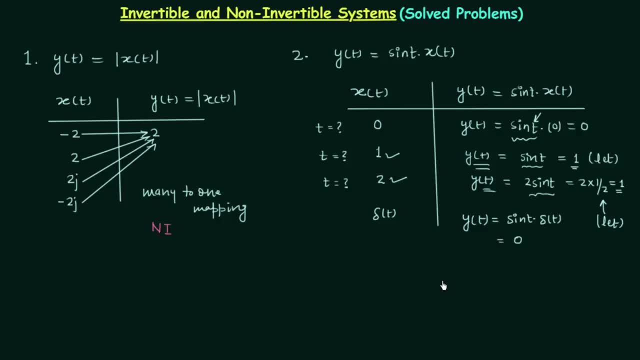 it is equal to 0?? I have used the property of impulse signal. If you remember the property, xt multiplied to delta t minus t1, it is equal to xt1 multiplied to delta t minus t1. Here t1 is equal to 0 because we have delta t. You can write it as delta t minus 0. So t1. 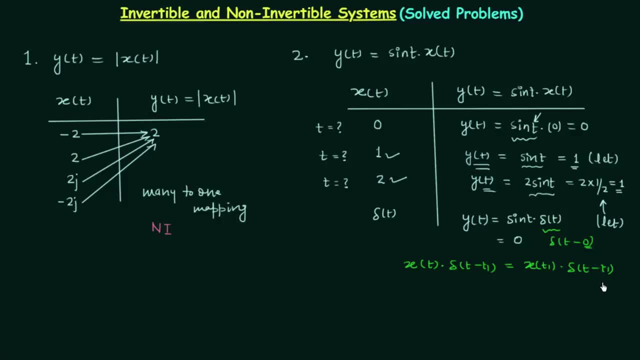 is equal to 0.. Put t1 in place of t in xt, The sin t is equal to 0. So you can write it as delta t minus 0. So t1 is equal to 0.. Put t1 in place of t in xt, The sin t is. 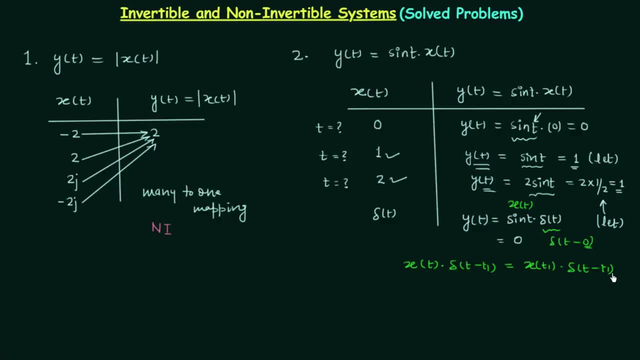 equal to 0.. Put t1 in place of t in xt. Put t1 in place of t. t1 is equal to 0.. So we will have x0 or sin 0.. Sin 0 is equal to 0.. So 0 multiplied by delta t is equal to 0. 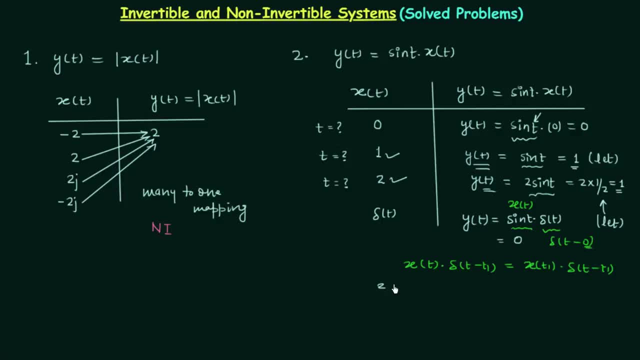 Now we will have twice of delta t. This will give us yt equal to sin t multiplied by twice of delta t. Again, we will use the same property. t1 is equal to 0. So we will put 0 here in place of t. So sin 0 will be 0.. 0 multiplied by. 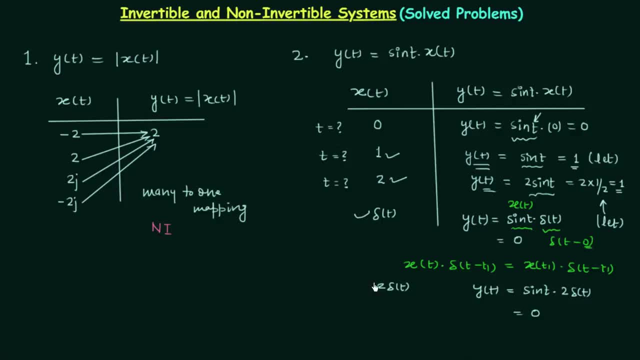 2 delta t will be 0.. So you can see, for two different values of input we have the same output And when this happens we know it is many to one mapping. Therefore the system is non-invertible. So I hope you now understand how to use the standard signals to find out. 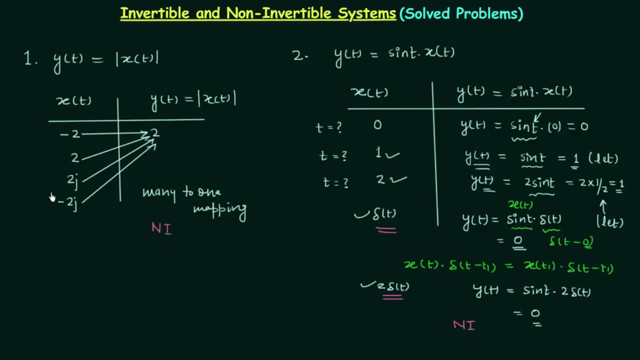 the answer when the question is like this. So let's get started. Let's get started. The question is little bit tricky. Let's move to the third problem. In the third problem, yt is equal to x2t. We will follow the same steps: Xt, yt. In the first column we will 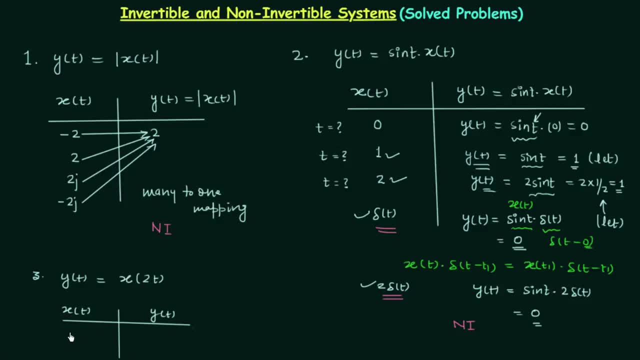 have different values of input In this problem also, I am not taking the numerical values, I will take the unit step signal yt, which is equal to x2t, will be equal to u2t. Now I will take minus ut, So yt will. 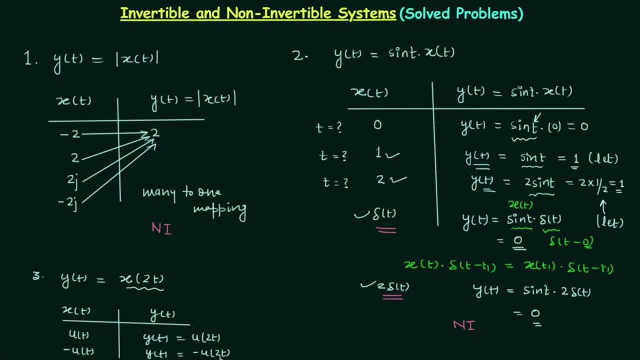 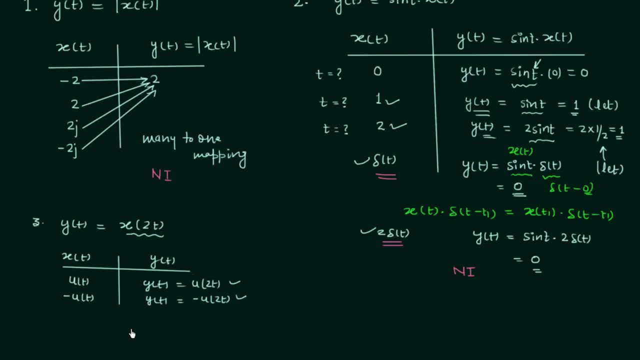 be equal to minus u2t. So you can see, for two different values of input, the output is also different. Therefore there is one-to-one mapping, And when there is one-to-one mapping, the system is invertible system. So this is all for this lecture, and now we will move. 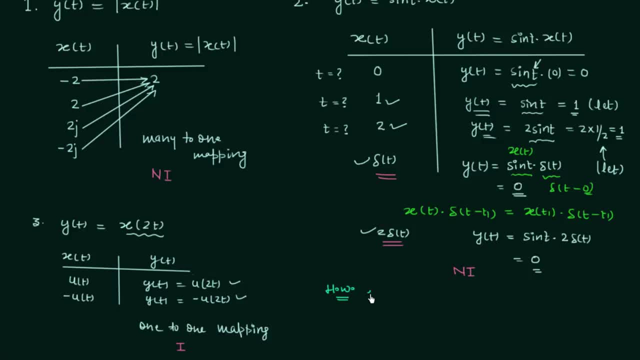 to the homework problems. In the first homework problem, Yt is equal to Xt square and in the second problem, Yt is equal to d by dt of Xt, and you are required to find out the nature of the two systems, whether they are invertible or non-invertible. Now, before ending this, 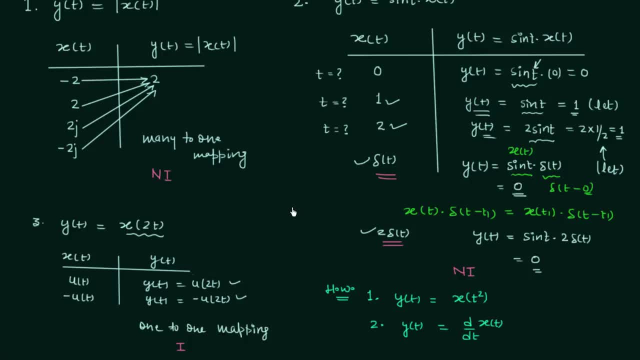 lecture. I want to explain two points which may confuse you. The first point is related to the use of this property and the second point is related to the process we have used in order to obtain different outputs in problem number three. I will start with the problem. 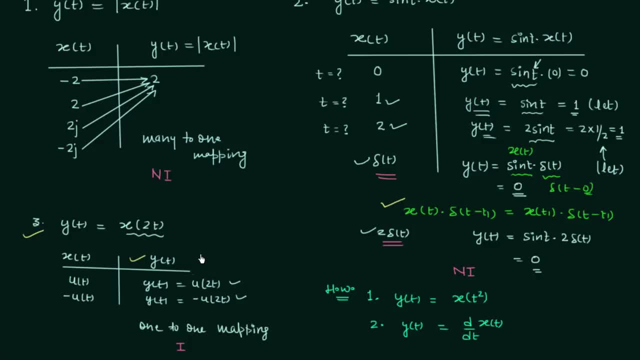 number three. You can find out the functionality of the system from the system relationship Here in the input is Xt given to the system whose property we need to find out, and the output of the system is Yt, which is equal to X2t. Now compare Xt and X2t, you will find there. 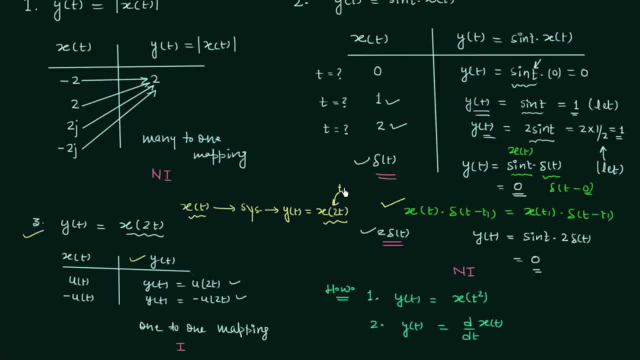 is time scaling. Two is multiplied here, which is the case of time scaling. So our system is performing the time scaling and we have the time scaled input. Now look at Ut. Ut is equal to Xt and the functionality of the system is to perform. 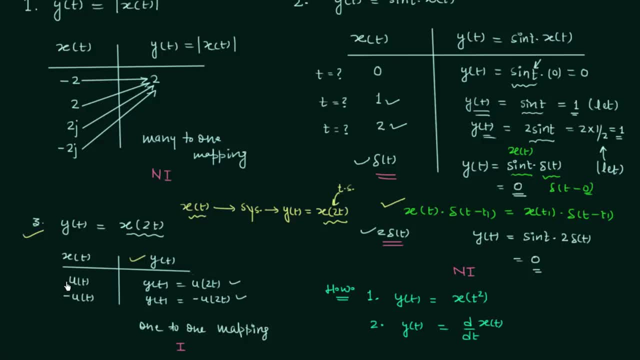 the time scaling. So our system will perform the time scaling on Ut by multiplying 2 to the time, So we have U2t. In the same way, when you have input equal to minus Ut, the system will again perform the time scaling and we will have minus U2t. So this is how. 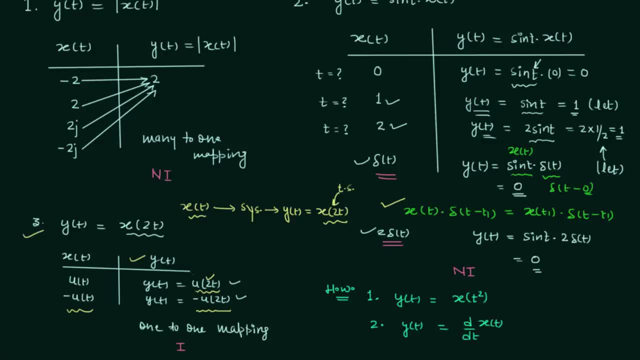 we have obtained the two outputs in problem number three. Now regarding the use of the use of this property, it is very simple. Xt, in our case, is equal to sin t and delta t minus 1 is equal to delta t. So delta t we can write as delta t minus 0. So if you compare, 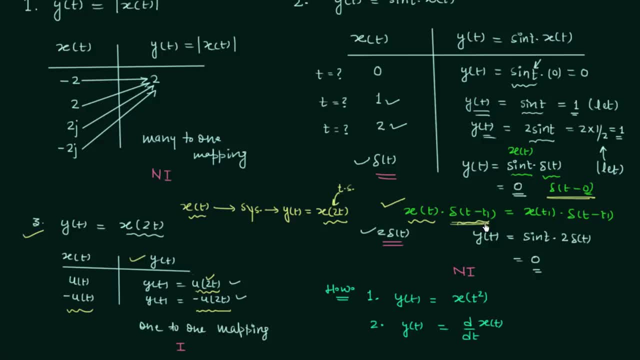 delta t minus 0. with delta t minus t1 you will get t1 is equal to 0 and it is equal to Xt1, delta t minus t1. So the impulse part will remain same. We will have delta t minus t1 here, which is same as delta t minus t1, but Xt will change to Xt1. So this t here.